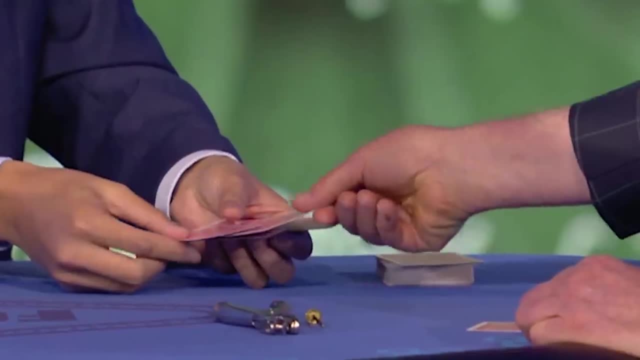 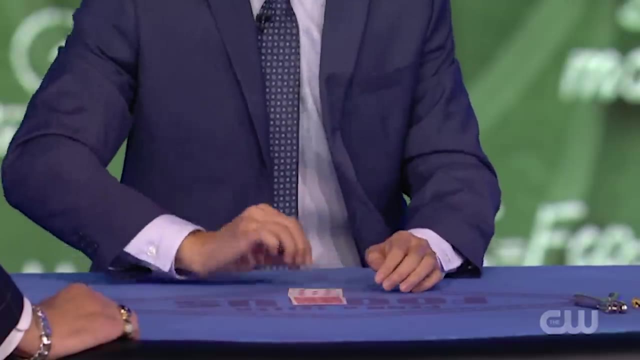 cards. Teller placed one of the red cards inside the black cards. He proceeded to place the second and third red cards. Stanley once again dropped the deck Again. the first three cards were red and the three black cards had traveled to the bottom. Stanley then moved on to explain that. 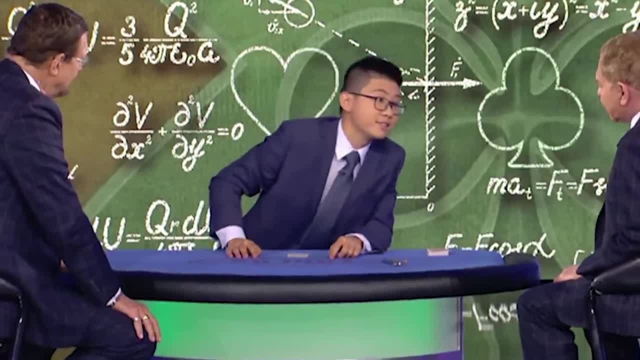 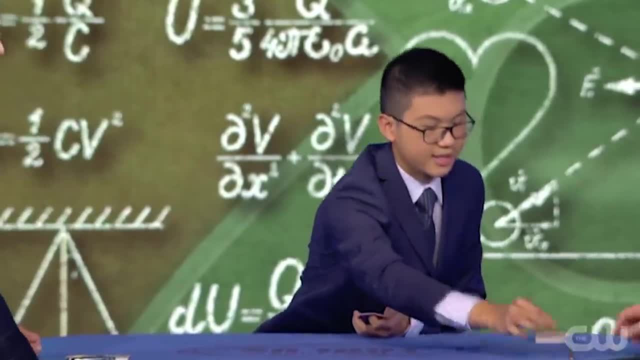 he may have used sleight of hand. so he said that he has invented a sleight of hand prevention machine. The first part is a hole puncher and the second part is a paper fastener. He gave the two tools to Penn and Teller for inspection. He punched a hole at the 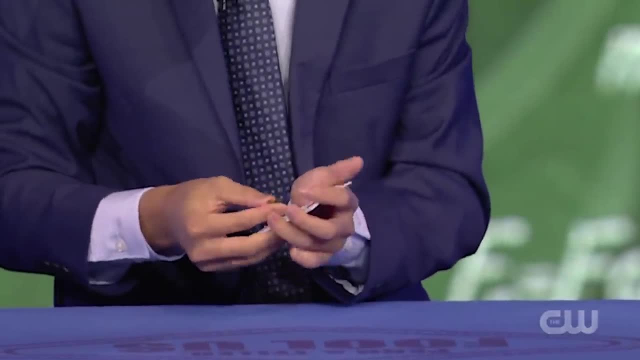 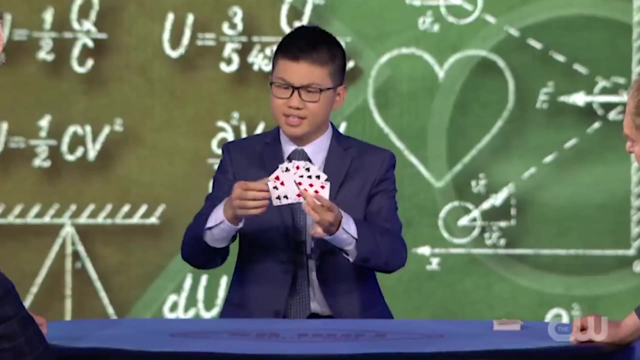 bottom of the cards. He used the paper fastener to hold the cards in place to prevent any sleight of hand. He showed that the cards are mixed in a red-black pattern and that, no matter where you turn the cards, the order cannot be changed because of the paper fastener. Stanley dropped. 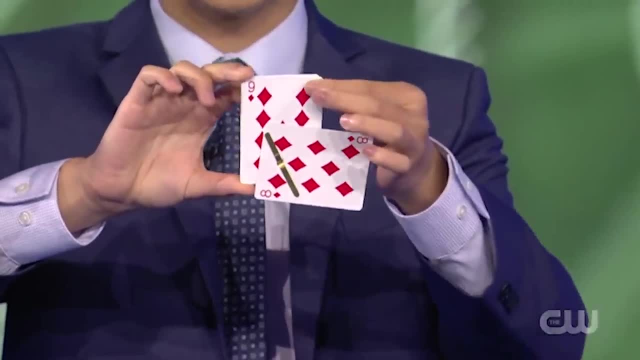 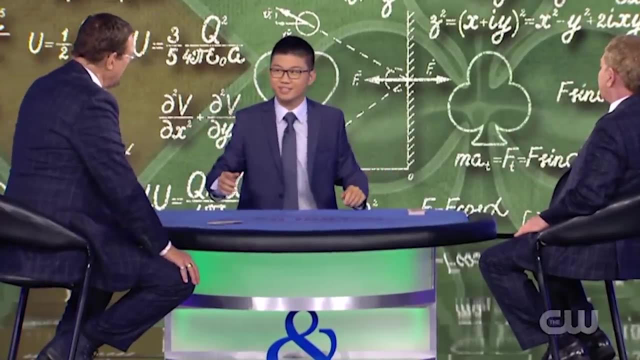 the cards on the desk. He proceeded to show the first three red cards and that the three black cards had magically traveled to the bottom. Stanley said that the trick has not ended and the real physical evidence that black ink is heavier than red will be proved by the control. 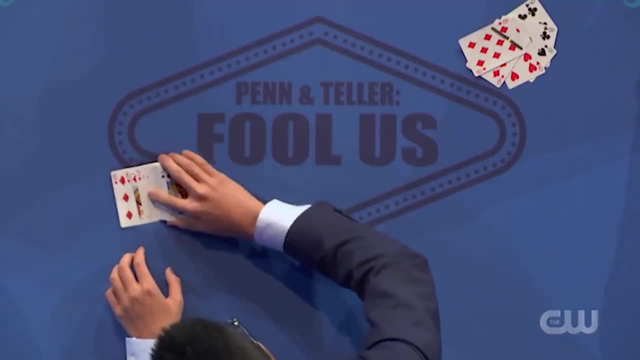 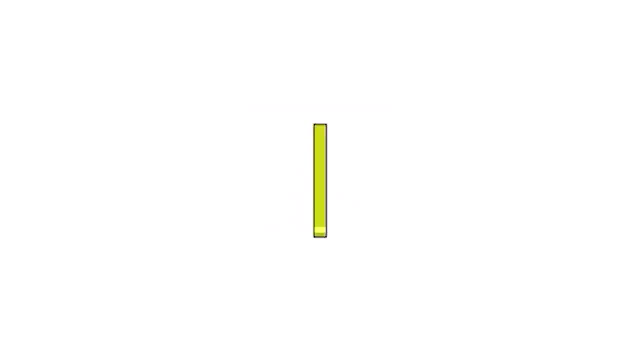 group. He dropped the deck On the deck, all the black cards traveled to the bottom of the deck and all the red cards stayed at the top of the deck. Spoiler alert: If you accidentally clicked on this video and don't want to know how such tricks work, I will give you 5 seconds to click off. 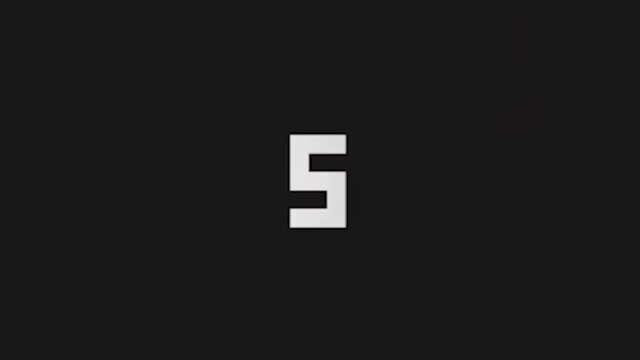 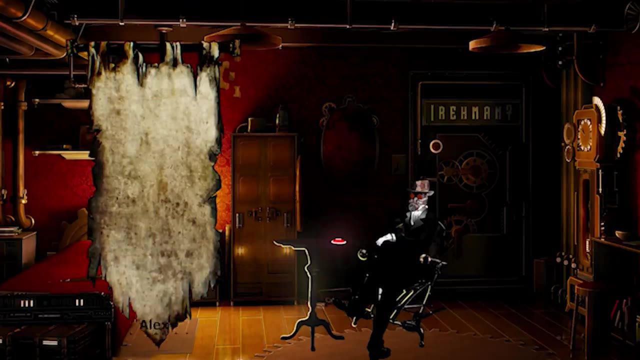 this video, but if you consider magic as a puzzle, then stay tuned. Now, before I get down to the reveal, I want to give a quick shout out to my wonderful patrons for supporting my work. Their support is a reason I am able to improve the quality of my work and I am able to improve 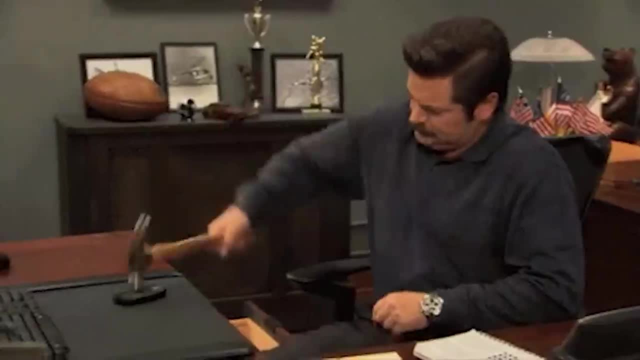 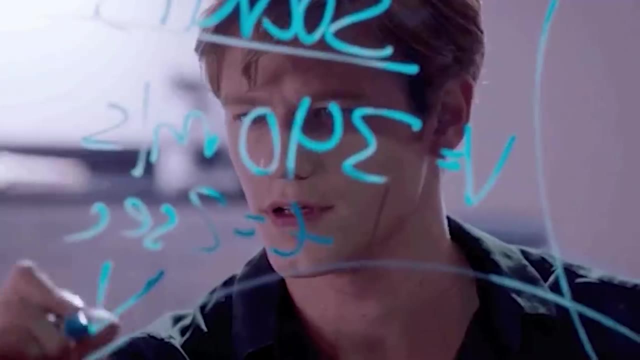 the quality of my work. I am able to improve my content and upload more regularly. We will break the trick into two phases. in the first phase, we'll discuss the observations and in the second phase, based on those observations, I will explain exactly how Stanley Joe performed. 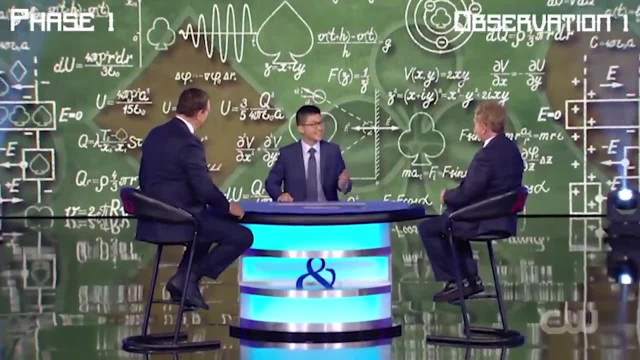 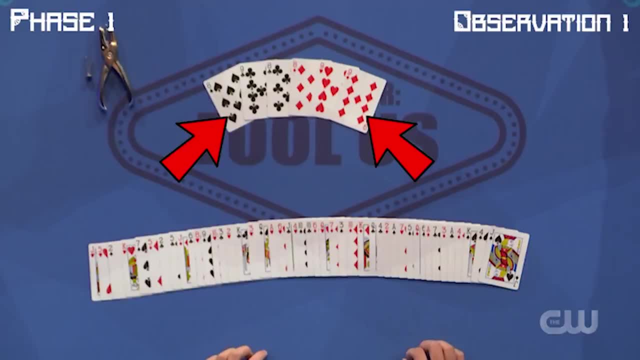 these incredible card trick. When Stanley initially started the performance. we can see that he has already spread the entire deck of cards onto the table and even spread the three blacks and the three reds he was going to use during his performance above the spread. 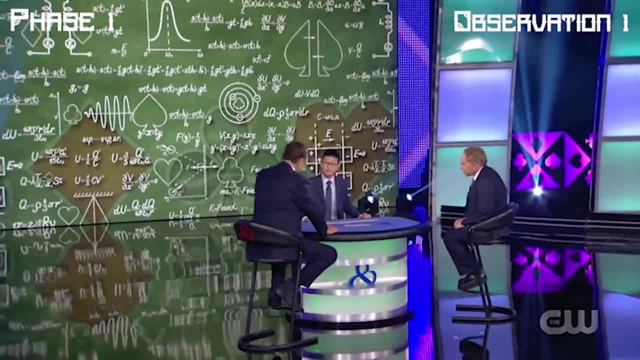 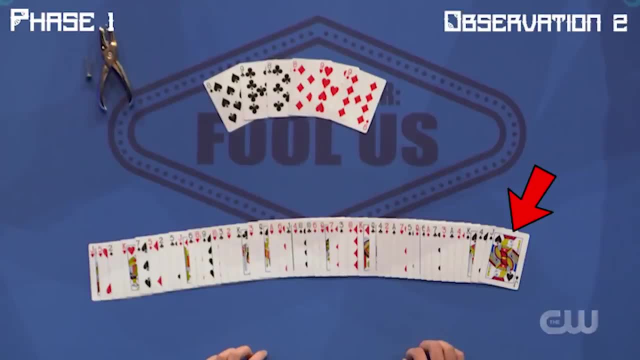 This point is very crucial in helping us figure out how Stanley's trick was going to be executed. The second thing I want to point out is regarding the spread. once again, you can notice that the top playing card in the spread is the jack of spades and the bottom card we can 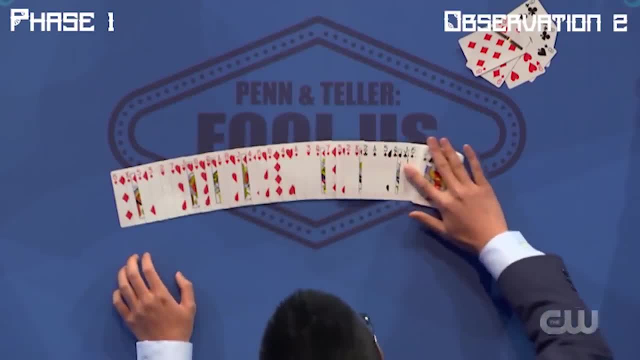 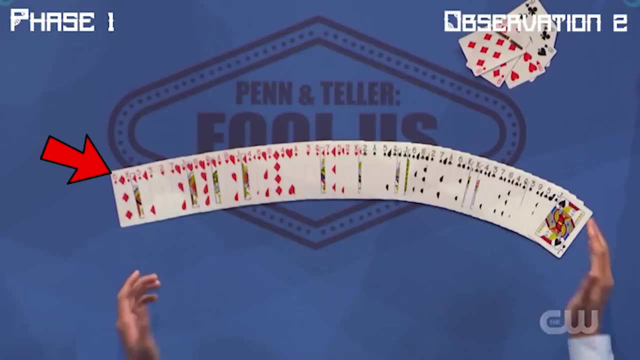 clearly see is the jack of hearts. But later in the performance, when the deck is miraculously organized into blacks and reds, the bottom card is no longer the jack of hearts, rather, for some odd reason, it is the six of diamonds. This clearly does not make sense, because he did not do anything fishy with the deck when. 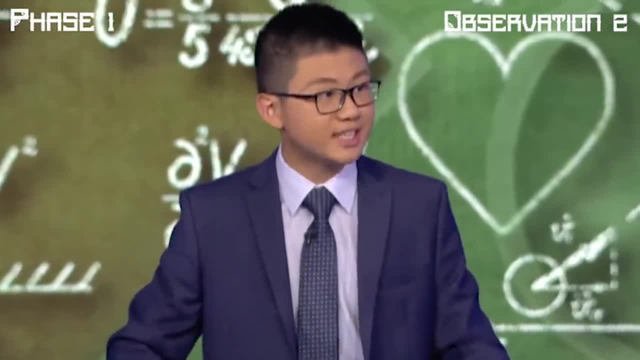 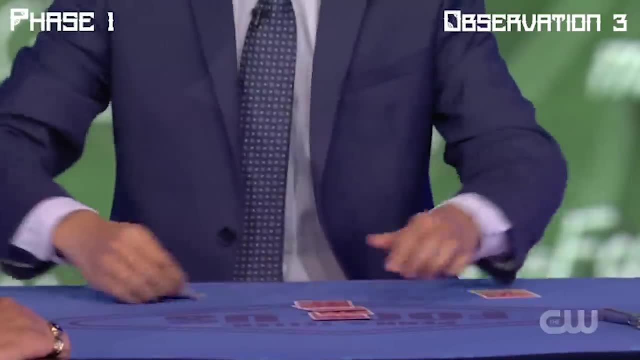 he closed the spread and placed the deck on his left side of the table. Now let's get into the video. After closing the spread, Stanley separated the blacks from the reds and, one by one, started to place the blacks and the reds alternatively on top of each other. 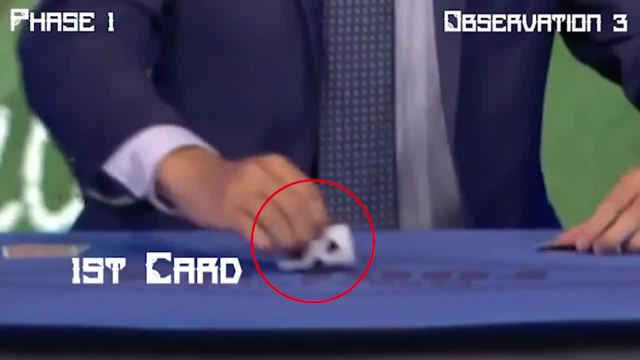 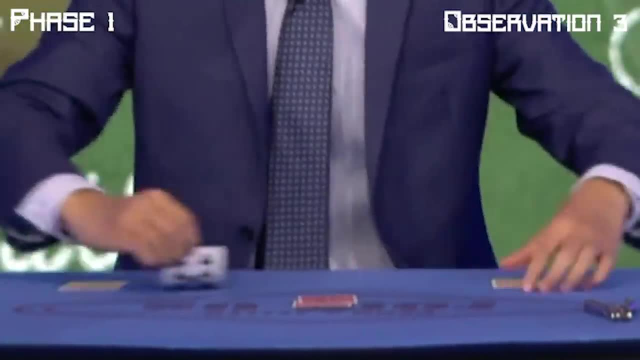 While doing so, we can see that for the first card from the black pile he does place a black card, but from the second red pile he does not flash which card he was placing as a second card. For the third card, he once again flashes: it's a black card. 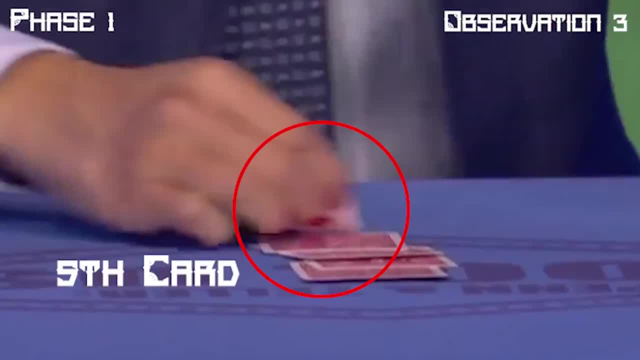 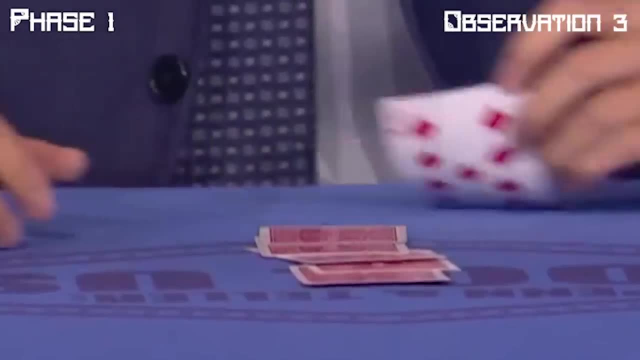 The fourth card he flashes as a red card. but for his fifth card, if we pause the video we can notice that it is not a black card, Even though it was in the black pile. And finally, the sixth card, he shows that it is in fact a red card from the red pile. 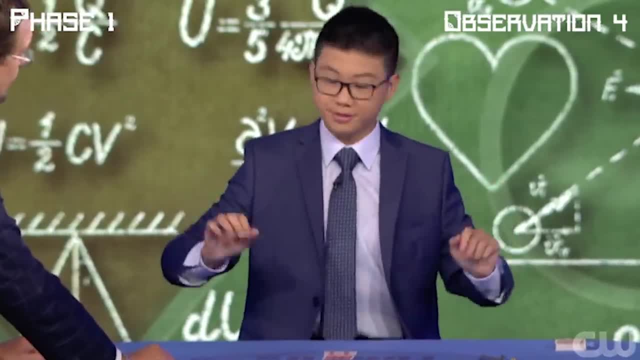 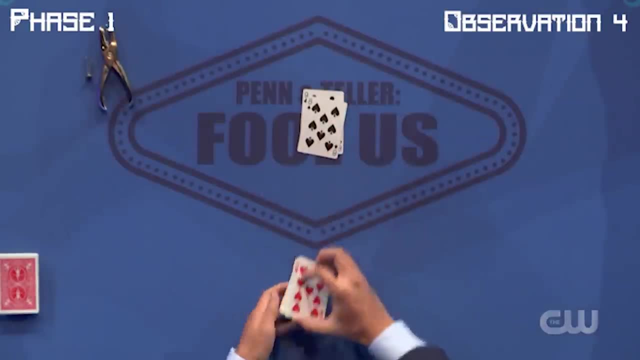 Another odd thing you will spot is after counting the red cards from on top of the packet, he does not do the same procedure with the black cards, rather picks up all three black cards and spreads them all together to display. And while picking up the red cards, we spot him separating the cards and changing their 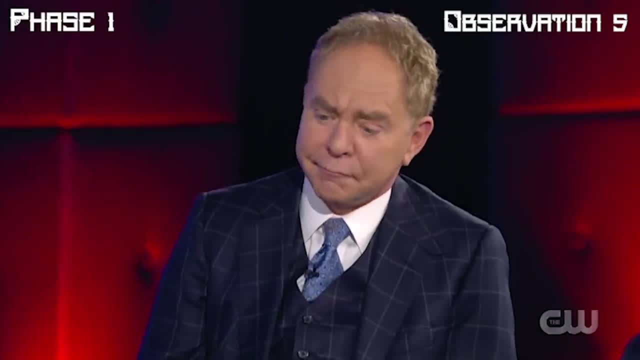 position right here at this moment. Then we spot a camera, cut during this moment towards teller by the editors of the show while Stanley was holding on to the black card And finally, the sixth card. he shows that it is in fact a red card from the red pile. 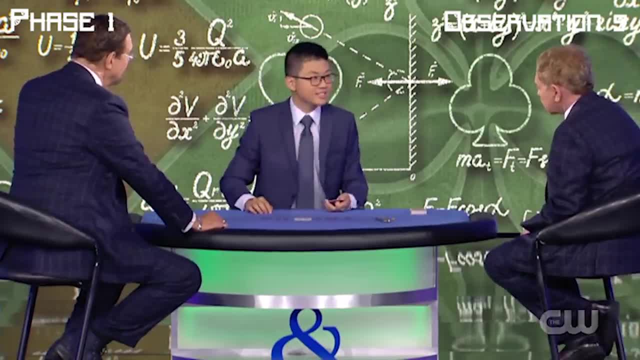 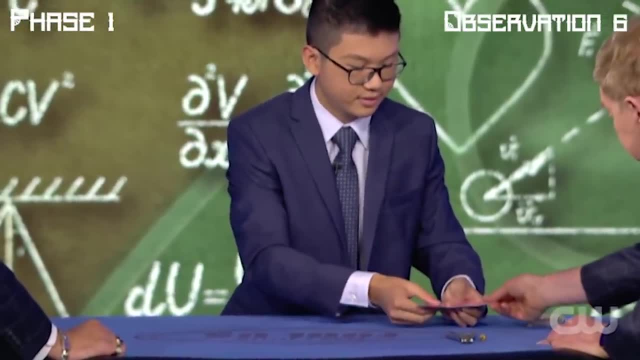 And while Stanley was holding on to the three red cards in his left hand. You will understand in the explanation why the camera cut was important. The moment Stanley asked teller to insert the red cards one by one in between the three black cards he was holding, we can spot the very top card, mistakenly flash a card right. 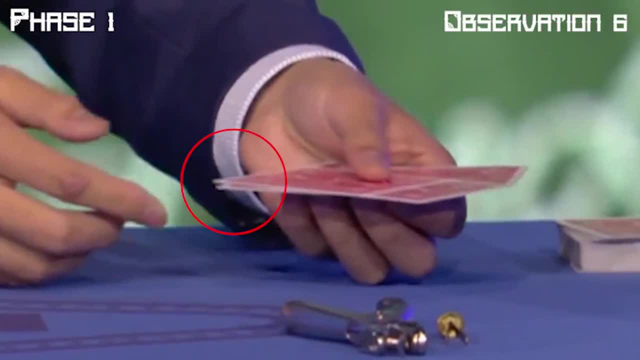 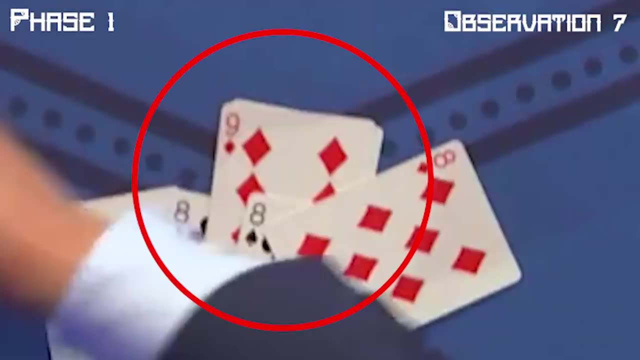 underneath it right over here, which means the very top black card, was a double card that Stanley was holding as a single card. Another moment we find Stanley flashing a double is when he is placing a red card between the black cards, and you can clearly see it right over here. 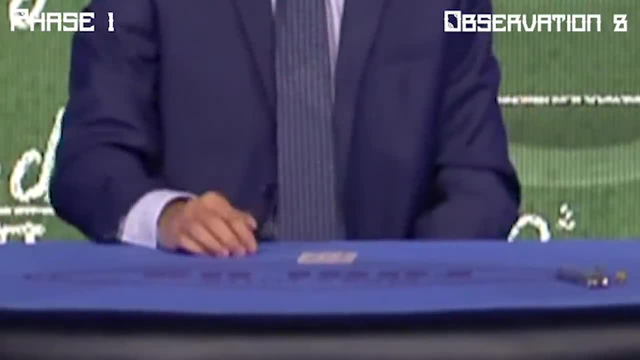 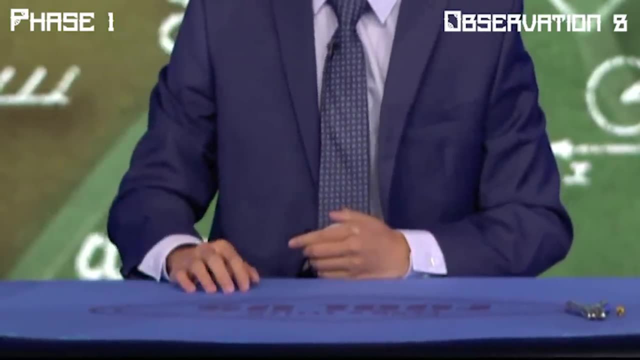 Finally, we spot Stanley putting his left hand behind the table while reaching for the packet of cards on the table with his right hand. We can conclude that the packet of cards that were on the table were switched with a packet that was behind the table. 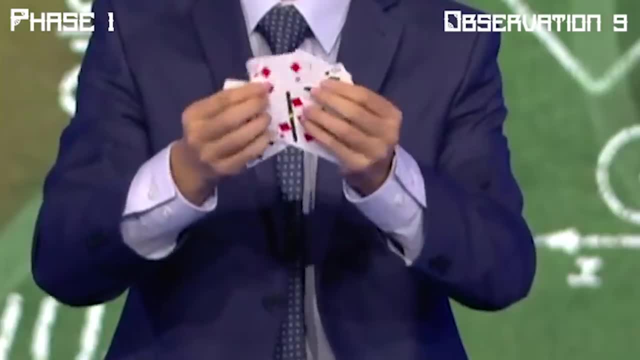 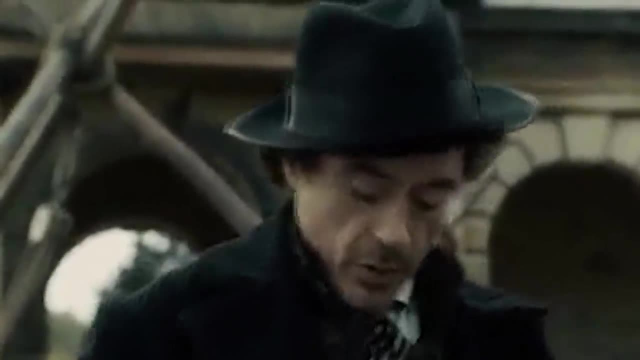 Finally, we spot Stanley doing a fishy rotational action while closing the fan of cards that he had fastened together with a paper fastener. If you haven't figured out how the trick works based on these observations already, I will now explain in detail how you can perform all the card tricks that Stanley did in his 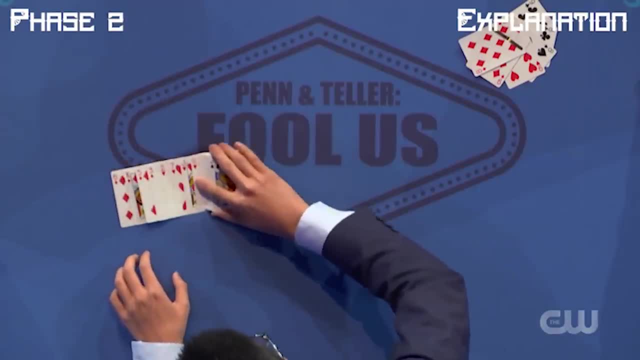 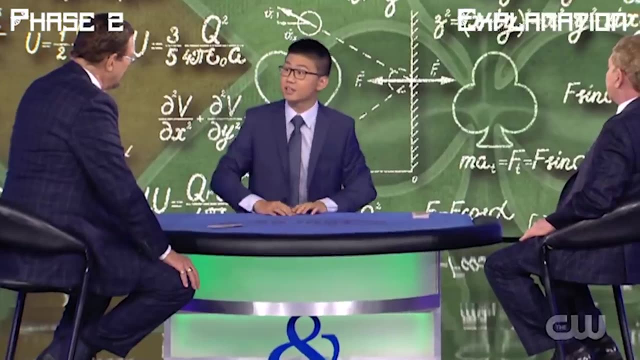 performance yourself. Let's start off with the easiest trick of Stanley's performance, in which an entirely shuffled deck of cards was separated into blacks and reds without any fishy movements. Well, the deck that Stanley was using was not an ordinary deck. rather, it was gimmicked. 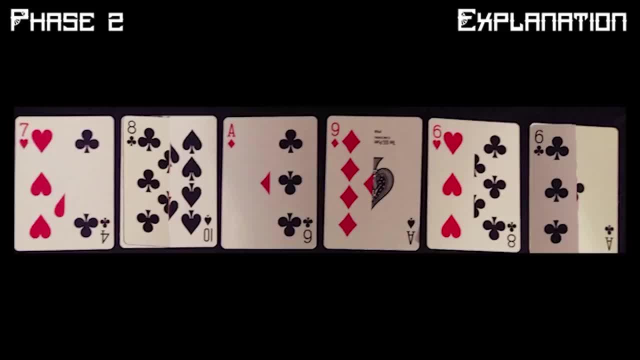 in a very clever way. For example, you can see that all of these playing cards are split faced. If we were to assort one half of the face playing cards in a sequence and spread the deck one way, it will show that the deck is in a sequence and by spreading the deck, the 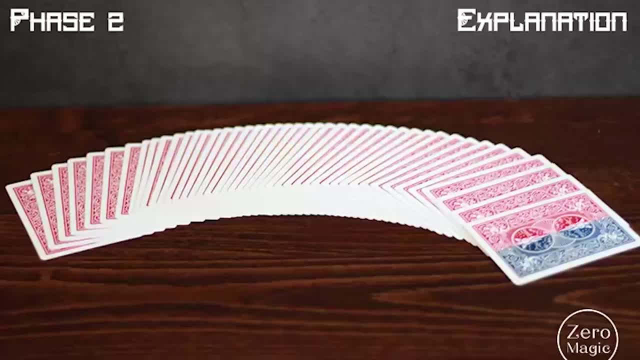 other way it will show that the deck is completely shuffled. A similar concept is used in a color changing red and blue bicycle gaff deck. You can see that when the deck is spread one way, it shows all the cards are red. but when 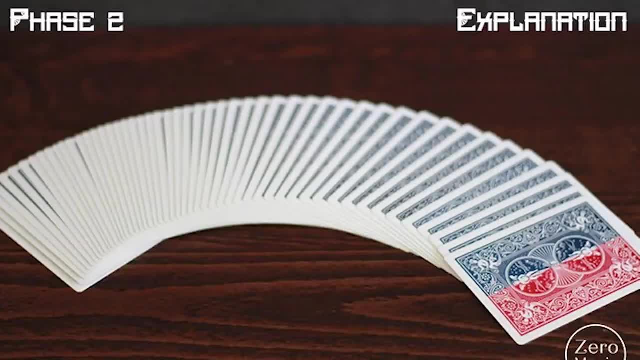 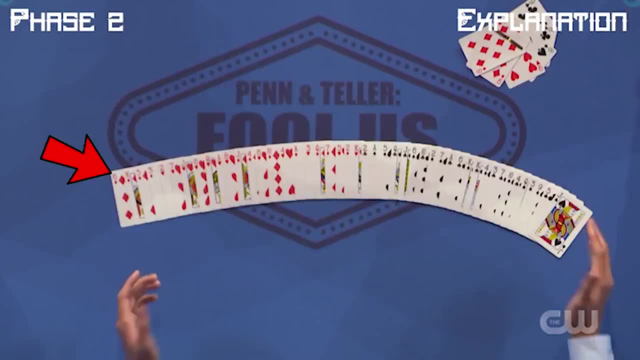 the same deck is spread the other way, it appears as if all the cards have turned blue. This is also the reason why the bottom card, which was the jack of hearts in the first spread, turned into the six of diamonds in the second spread, because the bottom card 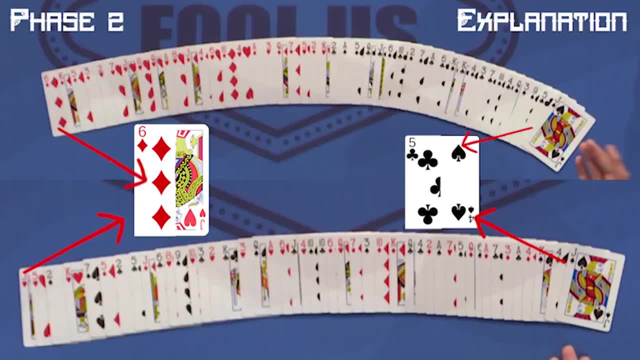 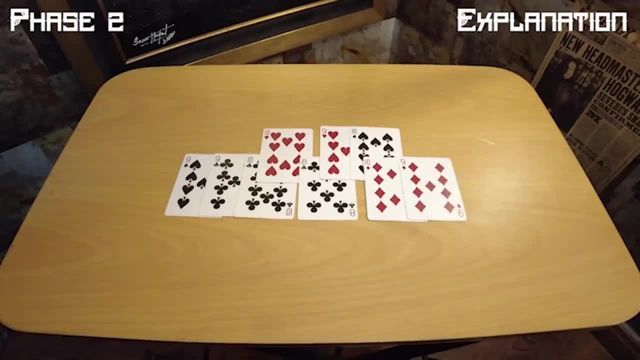 was a split face with a jack of hearts on one side and the six of diamonds on the other. The only card that wasn't split faced was the top card, which was the jack of spades. Now I will explain how to perform the remaining card tricks that he performed, in which he 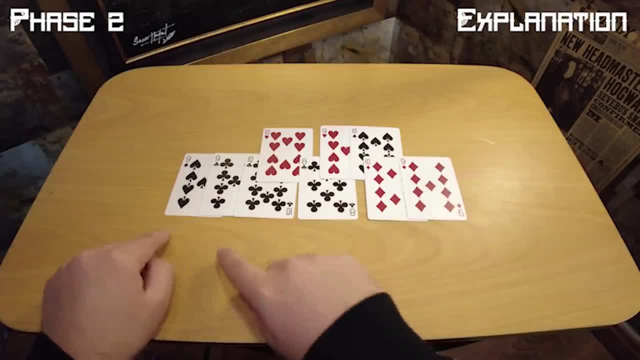 separated the three blacks from the three reds. Well, to perform the trick, you will need five blacks and four reds. You can use duplicates, for example, use two, nine of clubs. But for explanation purposes, I'm using the playing cards from a single deck because 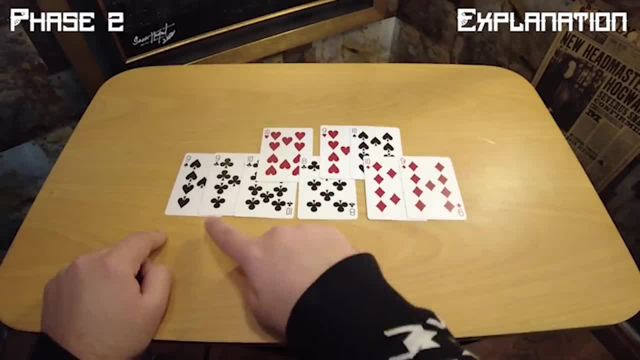 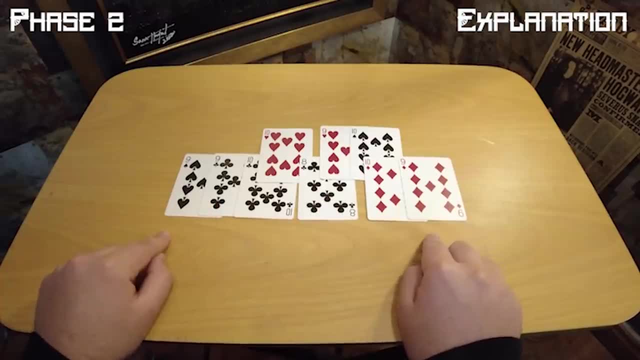 while performing, the attention is not given to the value written on the playing cards. rather, the only focus of the spectator is what colored playing cards are being used. You're going to organize the playing cards as you can see. You can see that the cards that are being played are the same as the cards that are 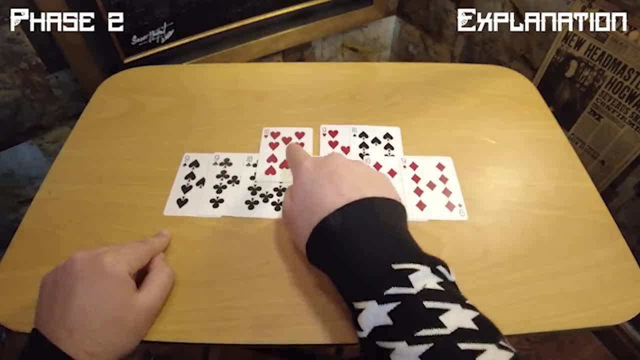 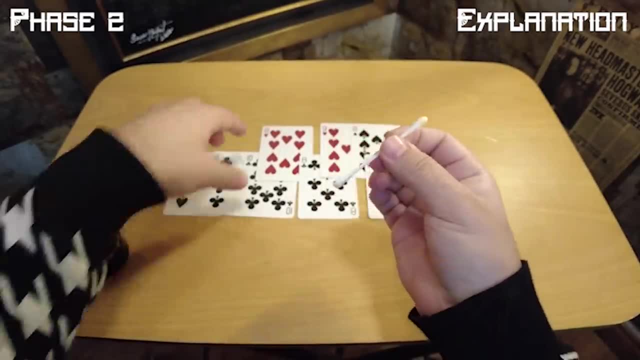 being played. These three outjogged cards will have a special adhesive known as octopalm anti-gravity gel. This gravity gel is rubbed on the very center of them using a cotton swab. For the first card, you will create a thin, invisible film on the face, and for the remaining, 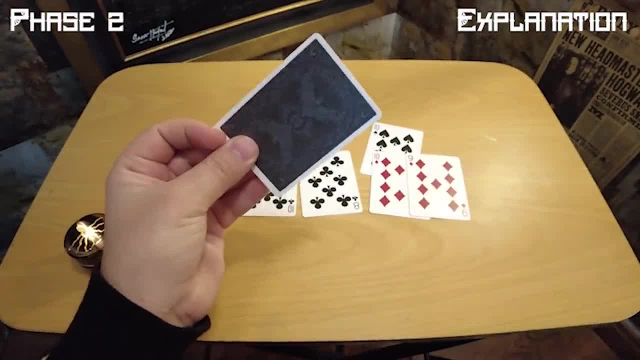 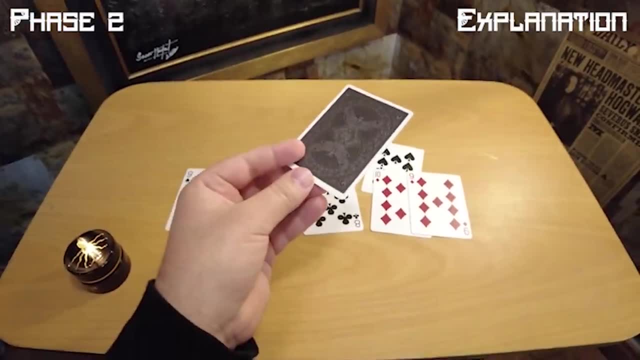 two cards. you will coat a small film at the center on the back of the playing cards. You can see that this invisible film is hardly visible at a distance and would not even be visible in most lighting situations. You are then going to square up these three playing cards so that only the nine of hearts 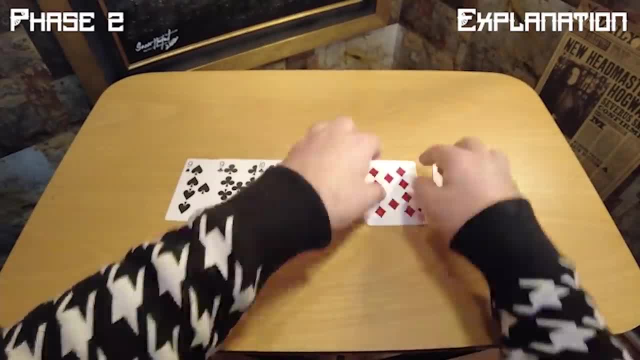 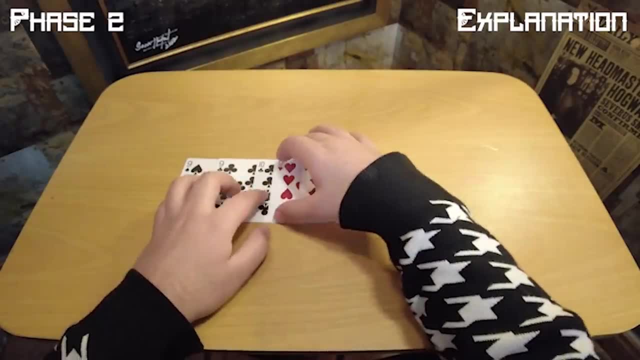 is visible from the top, and you're then going to square up these two cards, so only the ten of diamonds is visible from the top. This is the reason why Stanley already had the cards spread on the table, because the setup was designed in such a way that he would not have to worry about squaring up the cards. 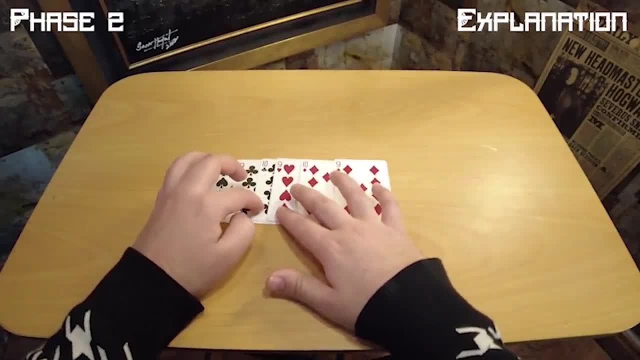 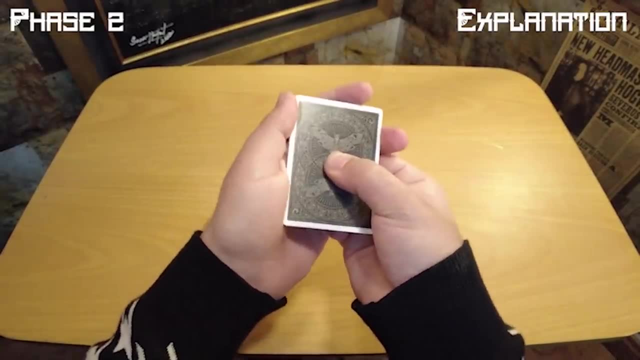 while spreading them. rather, he had already spread the cards, so he only would have to square them up. We are then going to flip over the squared up packet and apply light pressure so that the cards stick together. You are then going to count three cards from the top. 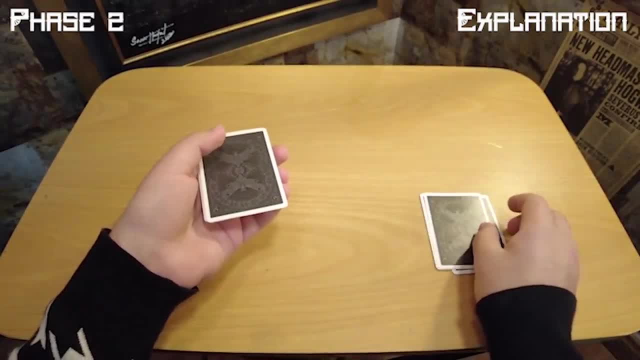 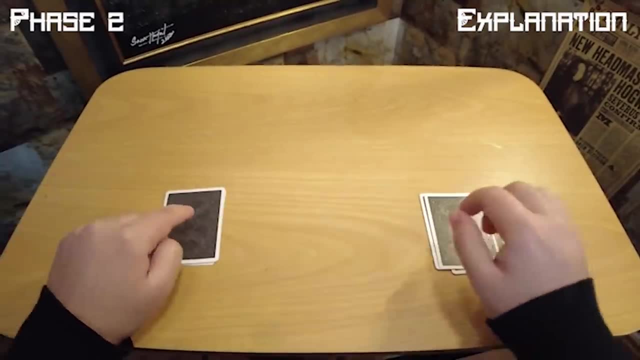 The first two cards are singles, Where the second card is going to be a double that will be stuck together due to the adhesive. The remaining three cards include a triple card on the very top and two single cards on the bottom. So the black packet is on your right side and the red packet is on your left. 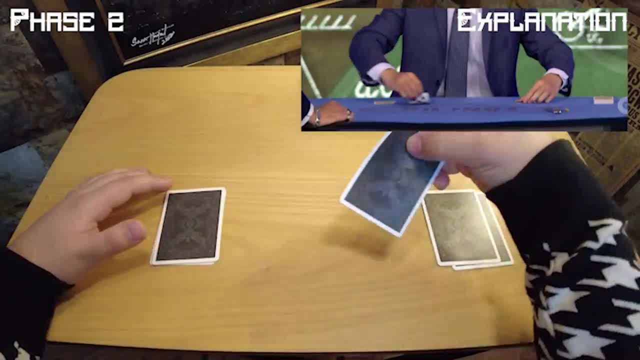 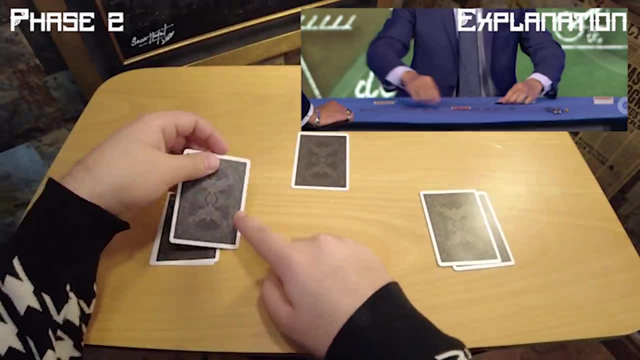 While placing the cards one by one and in alternating fashion, he placed one card from the black packet and slightly flashed it, which was a black card. The second card he did not flash. This is because the second card was a black card but was sitting on top of a red pile. 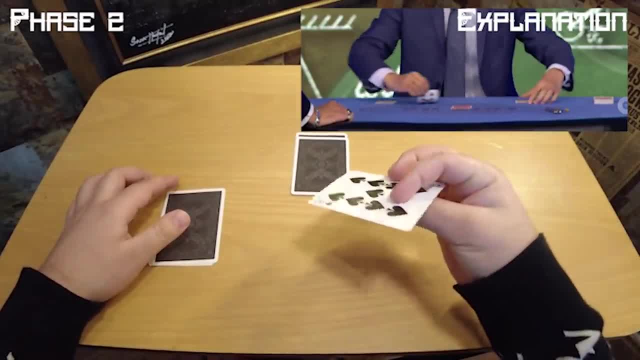 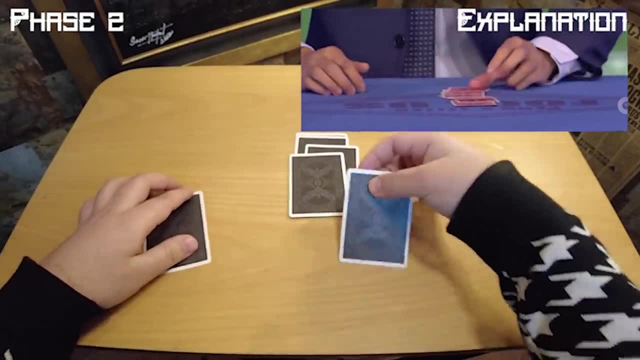 The third card was a black card he flashed in his performance. The fourth card is also a black card, But the fifth card is not a black card. it is in fact a red card which we also caught Stanley secretly trying to place. 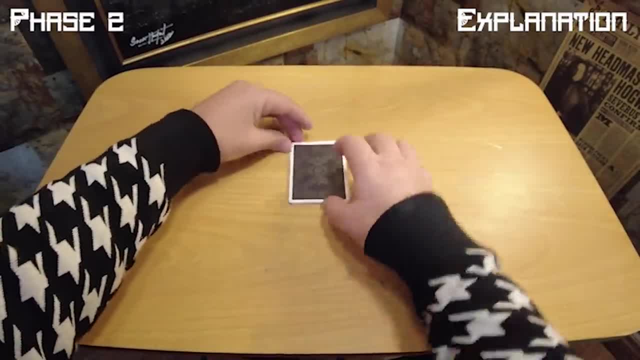 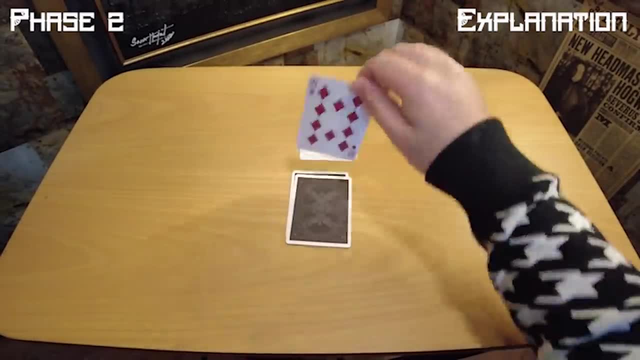 And finally, the sixth card is a red card. You're then going to square the cards up and drop them, And then start counting the cards one by one from the top, and you will see that the three reds are on the very top. 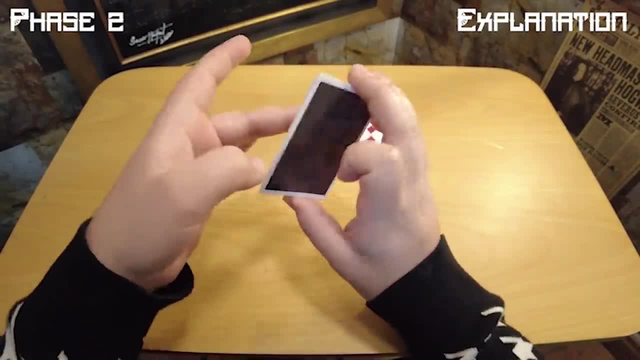 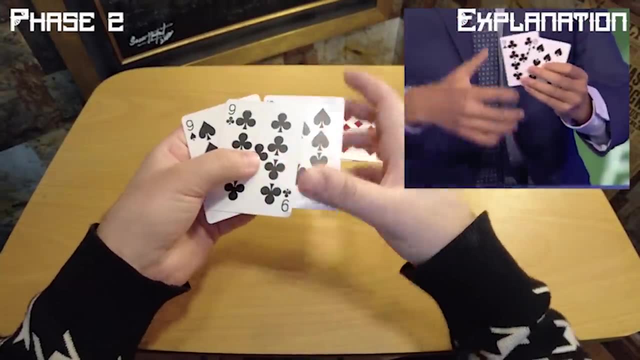 But to spread the three blacks you're going to peel off one card from the bottom and one card from the top and display it like this. So from the front perspective it looks like this: You are then going to place the triple ten of spades packet first on the table and the 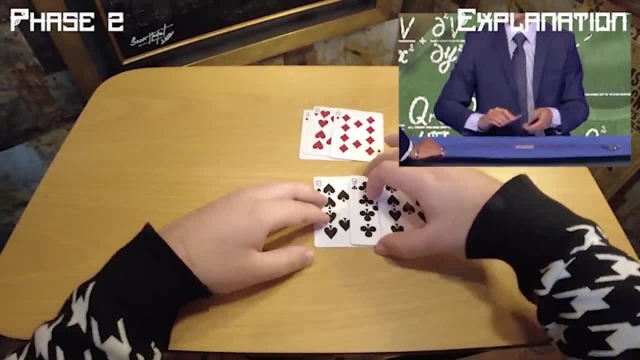 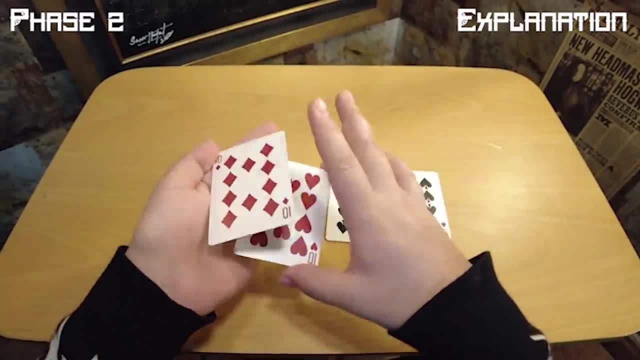 remaining singles on top of it. We then find Stanley separating the red packet and cutting it. at this moment, He actually strips out the double ten of hearts packet from between the two singles and places it at the bottom. This is because the ten of hearts packet has a black card stuck to the bottom of it. 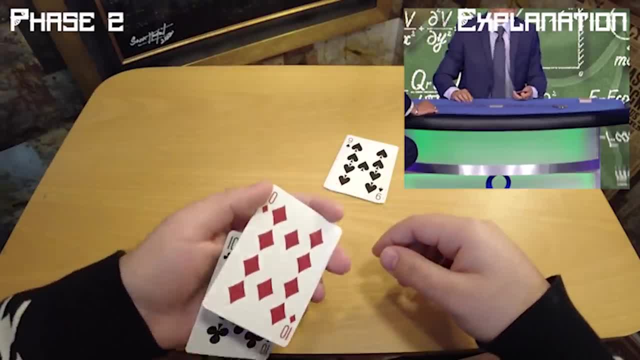 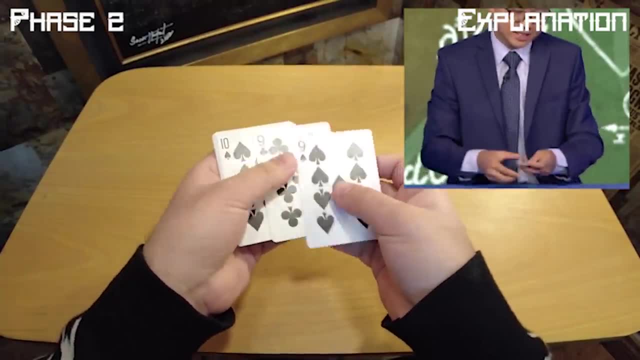 This black card is going to be ditched behind the table. While reaching out to grab the black cards, he ditches the single black behind the table and places these three on top. This is the reason why the editors of the show had cut this section from the performance. 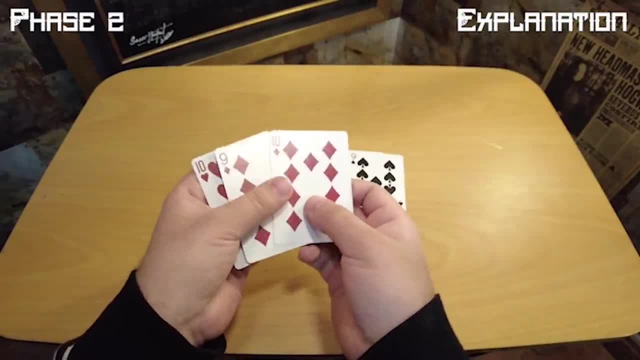 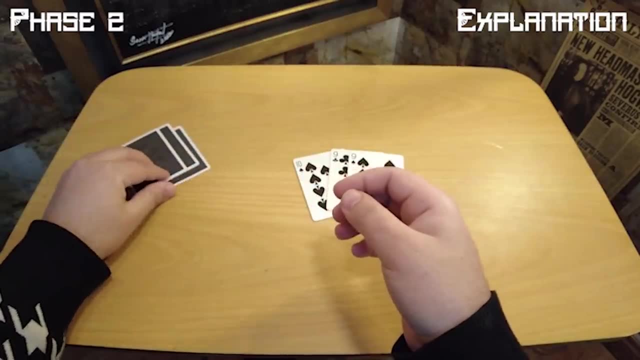 to hide the ditching moment that happened. Now the three red cards are examinable, And this is the reason why they were given out to Teller for examination, because no double cards were attached with the three red cards. You are then going to pick up the three blacks and flip them over. 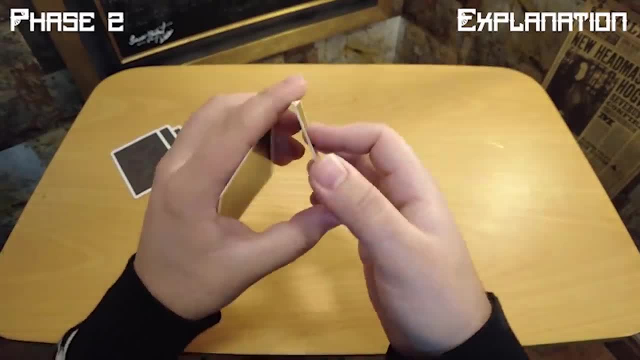 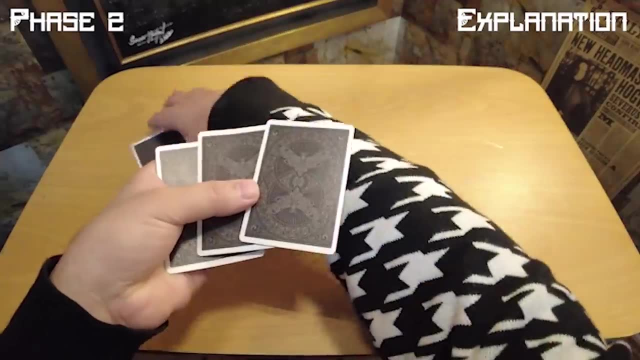 You're going to hold the two singles in a dealer's grip and separate a single card from this triple card from the bottom and hold it as a second card. This top card is a double playing card. You're going to place the red cards one by one. 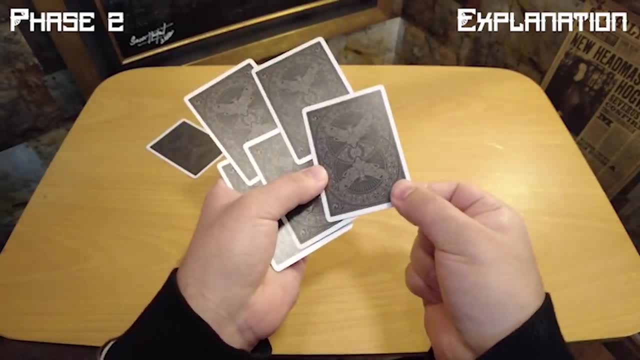 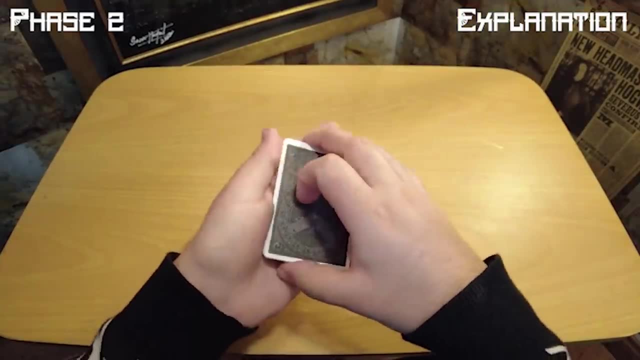 We noticed that while Teller was placing the second card, this card from here slipped out because it was a double card. And finally you're going to place the third card on top and square up the packet. After squaring up the packet, do the dropping motion and separate the reds one by one. 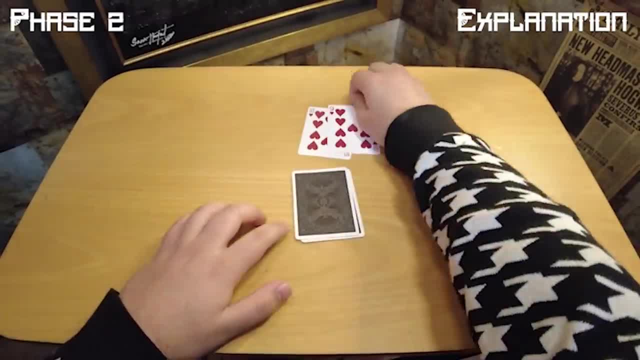 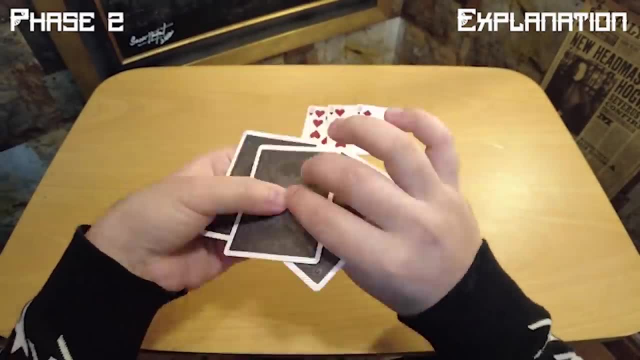 For the third red card, you're going to separate these two cards that are stuck together due to the adhesive, and this red card is a single red card. And finally, you're going to do the same spread that we did earlier to display the blacks. 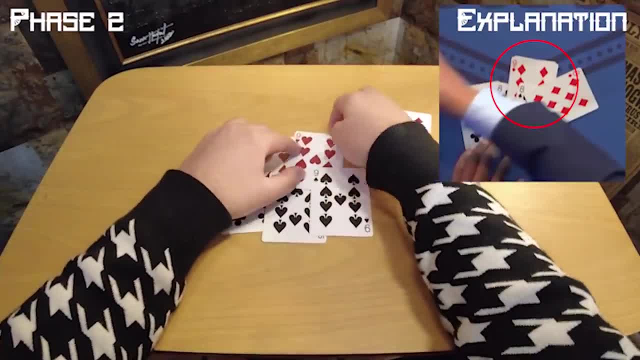 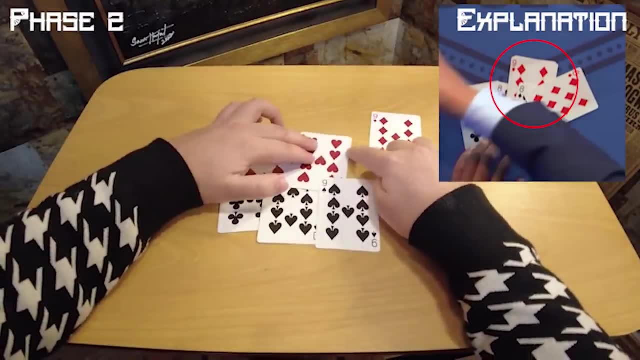 And then, while placing the reds back in between the three blacks, we caught Stanley flashing two cards. this is because this card has another card stuck behind it, which is a black card. After performing these two phases of separating the red from the blacks, we spot Stanley switching. 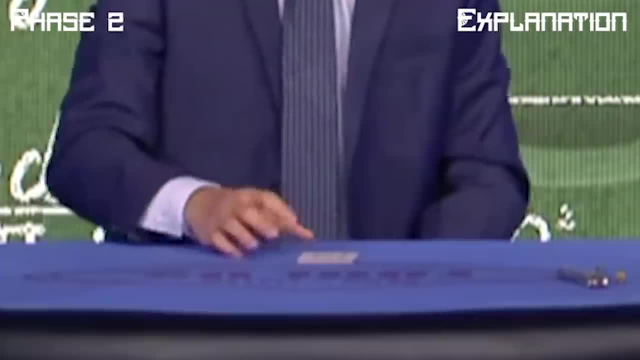 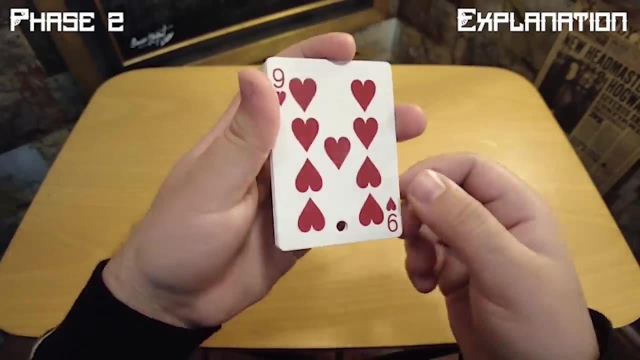 this packet for a second packet behind the table. This is because the second packet does not contain any doubles, rather only has three blacks and three reds. He then hole punched all six of the playing cards with the hole puncher and fastened them together with a paper fastener. 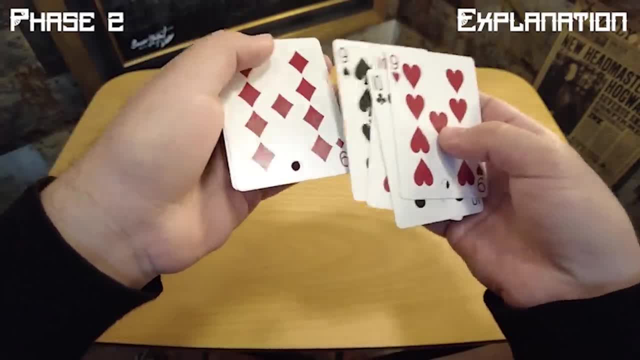 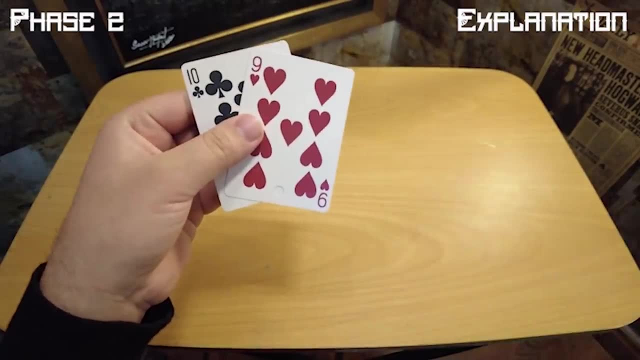 You can see here blacks and three reds that i have hole punched. before i explain the actual method of this trick, i want to clarify a misconception that many may assume: how the trick may be executed. this misconception is the fact that many believe the cards can change their position by some.